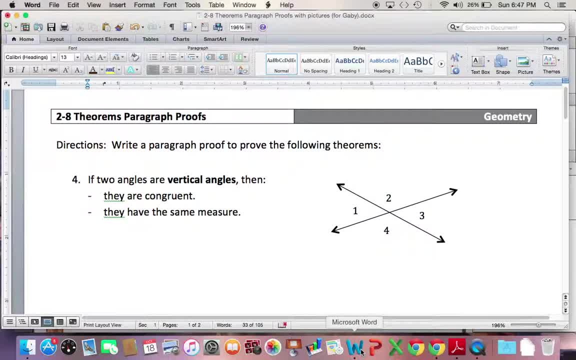 So let's go ahead. Let's go ahead and move on to your packet. So you'll notice that I'm starting at number 4 here. The first three proofs or, excuse me, the first three theorems from your packet are called right angle theorems. 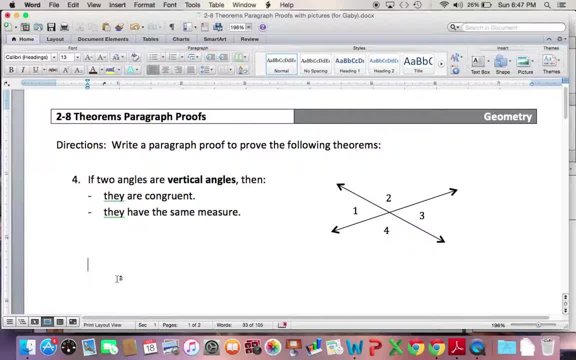 That's how your textbook refers to them, on page 155.. And we are not going to prove these three together because, based on your prior knowledge, they seem kind of obvious. So if today, once you're done with your homework, classwork slash homework if you've finished. 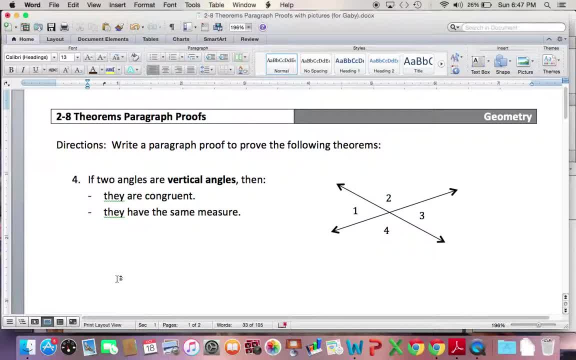 early. you will go back and prove these. If you do end up proving them, my suggestion to you is to forget about your prior knowledge and think back to your definitions, and you need to clearly state how you're going from one thought to the next. 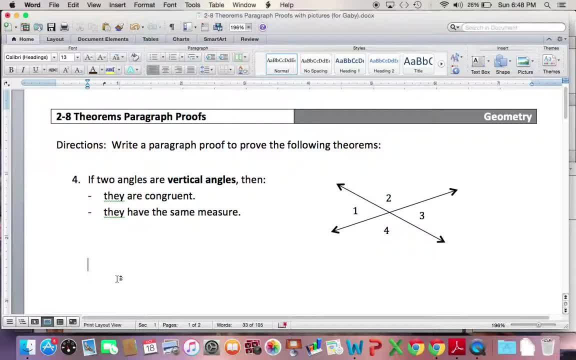 So they are a little bit more challenging, because the more obvious it is to prove, the harder it is to create that logical thinking. But it is possible as long as you know, you define, use your definitions and state clearly how you're going from one thought to the next. 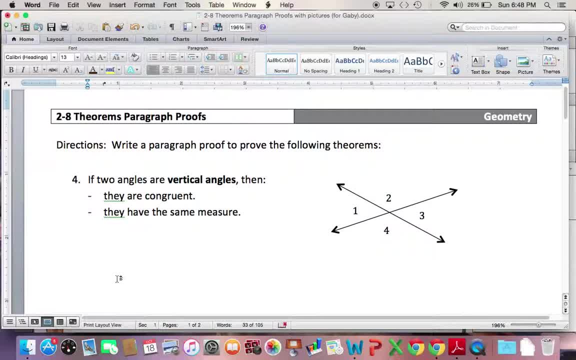 the next. Okay, so earlier last week you were assigned two paragraph proofs. We didn't really get a chance to go over them, and the reason behind that is because I wanted to talk about them further today and we're actually going to use those two to start our lesson on paragraph. 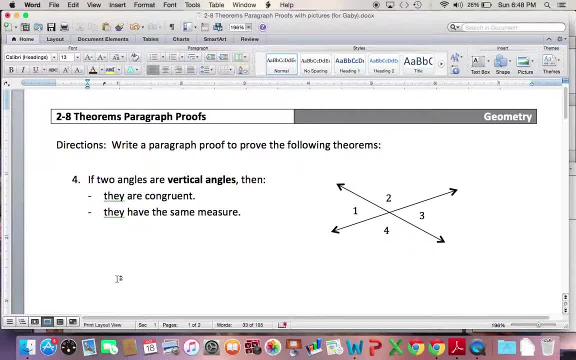 proofs. So go ahead and please flip to number four if you haven't done so already, So notice. number four states: if two angles are vertical, then they are congruent and have the same measure. So remember from our first lesson on proof writing: we needed to draw a picture that represents the 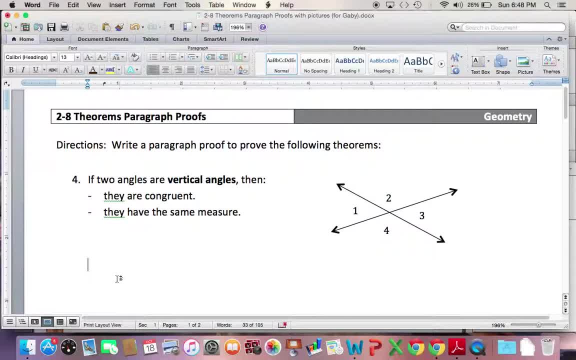 problem, and then we have to change our if then statement into what we're given and what we're trying to prove. So you'll notice I already have the picture over here. Let me give you a second or two to go ahead and draw that picture in. We're going to then write our what we're given and what. 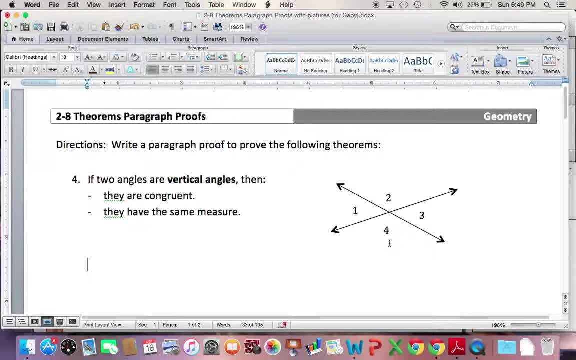 we're trying to prove, specifically based on our picture. So if you haven't drawn that, go ahead and draw that picture in, Okay. so next we need to state what we're given based on this. if then statement and what we're trying to prove, So let's go ahead and do that. We're given that angle one and angle three form. 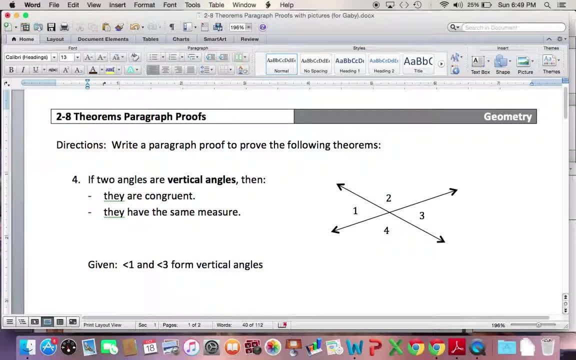 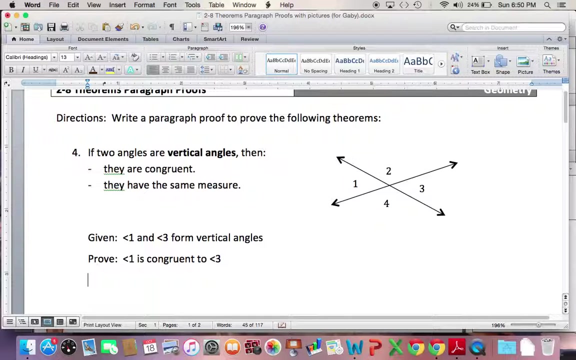 vertical angles. So we're just taking what we're given our if, then statement our hypothesis, and we're changing our hypothesis into our given based on our picture. Then we're trying to prove that angle one is congruent to angle three. and you guys, can you know, go ahead and write. 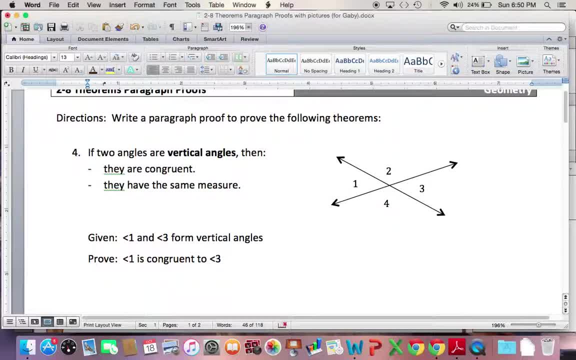 your congruency symbol. It's a little bit more challenging for me to find that on word while I'm going through this, so I'm just going to type everything out. But you know, you can use your little squiggle with the equal sign to state congruence. That's fine. And then the other thing. 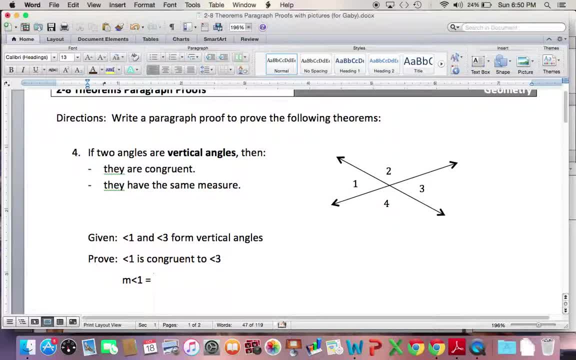 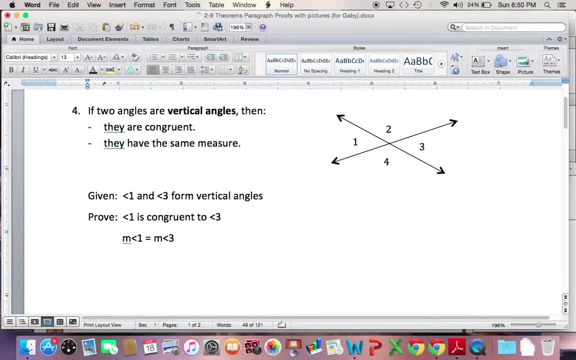 we need to prove is that measure of angle one equals the measure of angle three. So before going on to prove this, we need to kind of come up with a game plan. We want to think about what we're trying to do first. So remember, we can't use vertical angles are congruent, because that's what 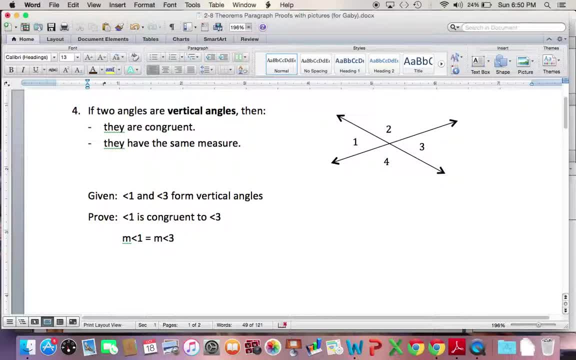 we're trying to prove. So we need to go about this another way and we're going to use linear pairs to do that. So let's go ahead and start. So remember, we can say it is given, it is given from the picture, that angle one and 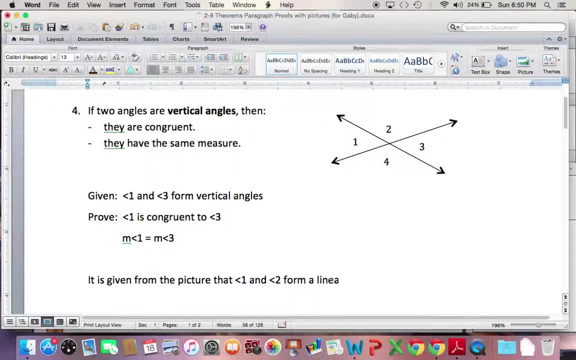 angle two form a linear pair. We know, since linear pairs imply supplementary angles, that the measure of angle one plus the measure of angle the measure of angle two equals 180 degrees. So we also know. so. from our picture it is also given. So we see the angle three, angle one minus two, tidy over two degree. 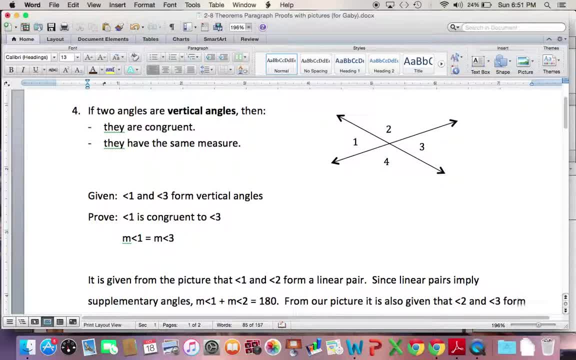 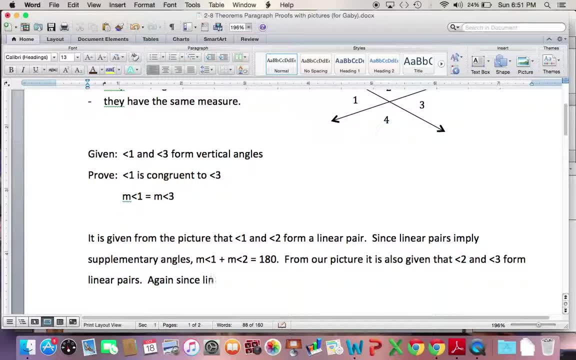 and angle one plus two and angle three, That is, ANGLE two and ANGLE three form linear pairs, screened again, since linear Pairs imply supplementary angles And We can say that the measure of angle, measure of angle two plus 2 plus the measure of angle 3 equals 180 as well. 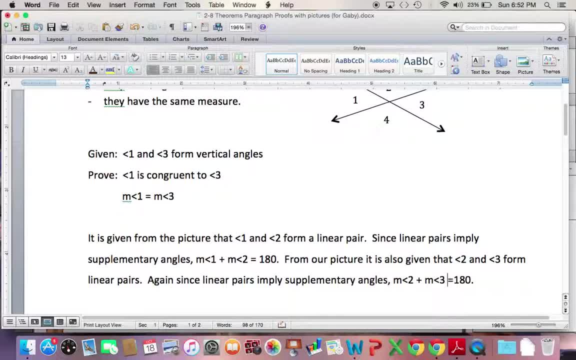 So now that we have these two angles, both angle 1 and angle 2, that are linear pairs, therefore supplementary, and angle 2 and angle 3, that are linear pairs and therefore supplementary, what we can do is set these two expressions equal to each other, since the measure of angle 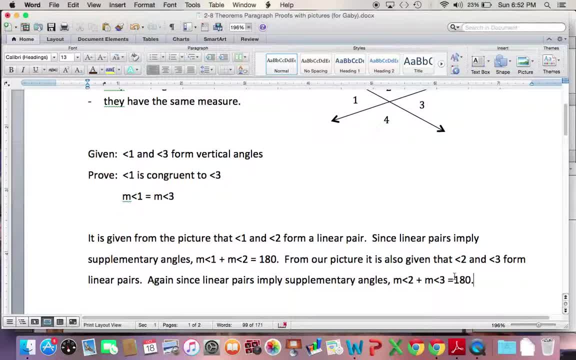 1 plus the measure of angle 2 equals the measure of angle 2 plus the measure of angle 3, we can say that those two are equal to one another. and then you'll notice you have the measure of angle 2 on both sides that we can go about canceling out, and then we're left with the 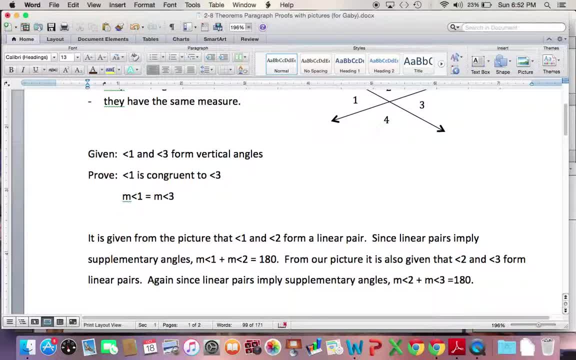 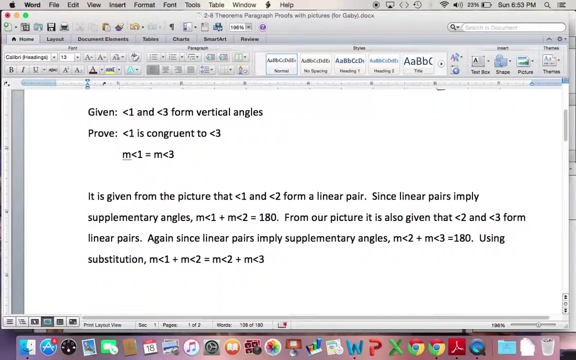 measure of angle 1 equals the measure of angle 3.. So let's continue writing this out. So, using substitution, we can set those two expressions equal to each other, that the measure of angle 1 equals the measure of angle 2.. So again, we're just setting those two equal to one another because we know they both equal. 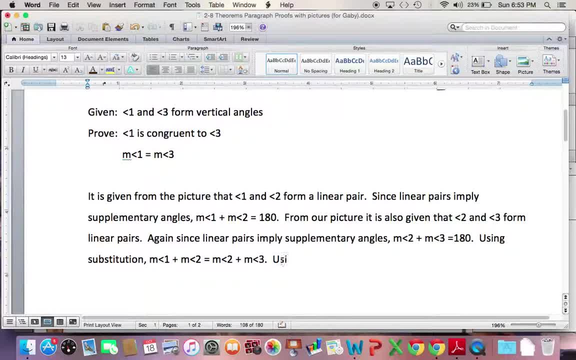 180.. So then, using the subtraction property of equality, we can set those two expressions equal to one another. So let's do that again. So we're gonna do the subtraction property of equality. we can say that the measure of angle 1 plus the measure of angle 2, minus the measure of angle 2, and I'm just going. 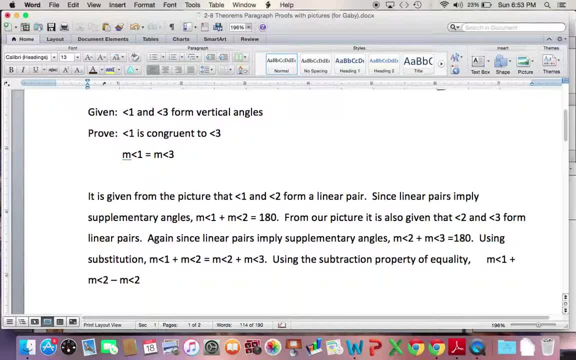 to space this out so you can see it all next to each other. It might be a little bit easier to kind of understand what's going on if you see it that way. So okay, now we all have it on the same lines. so the measure of angle 1 plus the measure. 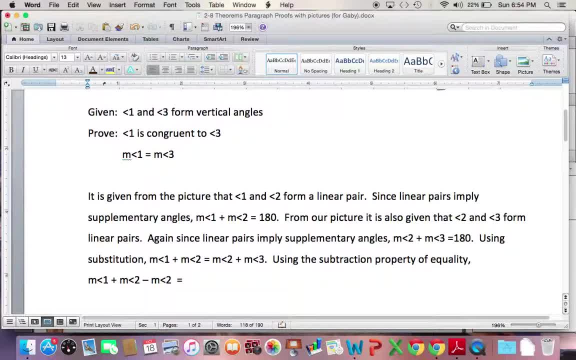 of angle 2 minus the measure of angle 2 equals the measure of angle 3.. So we've done that of angle 2 minus the measure of angle 2 plus the measure of angle 3.. So we're just subtracting the measure of angle 2 from both sides and you'll notice that both 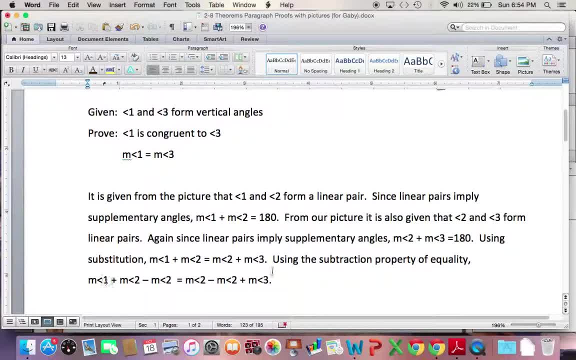 measure of angle 2s cancel on both sides, and you're just left with measure of angle 1 equals the measure of angle 3.. So then we can say, using substitution or simplification, whatever makes more sense to you, the measure of angle 2 cancels on both sides, resulting in the. I guess we can. 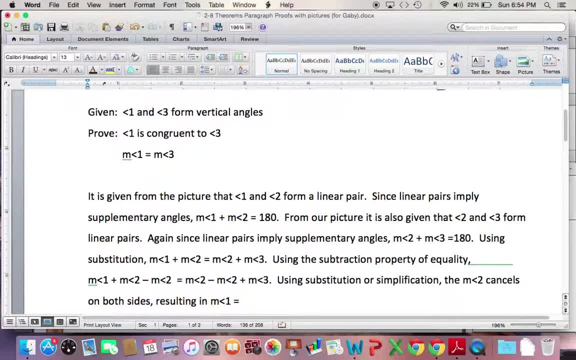 just say, in measure of angle, 1 equals the measure of angle 3.. Okay, So now we've proved that, one of the two things we're trying to prove. We proved that measure of angle 1 equals the measure of angle 3.. 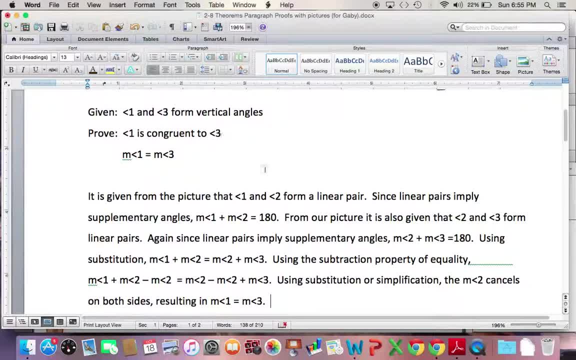 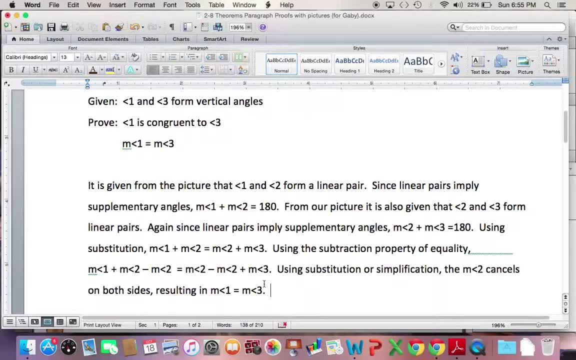 But now remember, we're still trying to prove the measure of angle 1 is congruent to angle 3.. So we need to switch this equality statement using the definition of congruence, to get the measure of angle 1 is congruent to the measure of angle 3.. 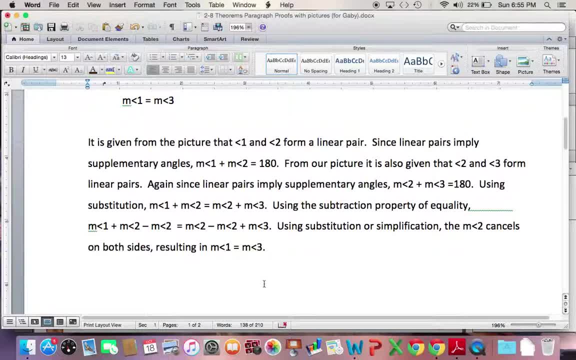 So, okay, let's go ahead and finish this up So we can say: furthermore, Using the definition of congruency, if two angles share or have equal measures, then those angles are congruent. So now we can say: angle 1 is congruent. again, you can use the symbol to angle 3.. 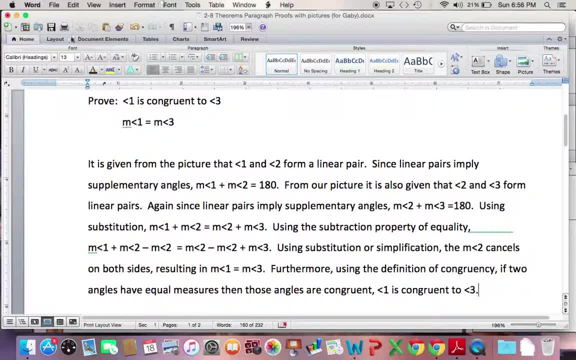 So now, looking back, we just want to make sure we've proved everything. We've proved 1 is congruent to 3, and we've proved the measure of angle 1 equals the measure of angle 3.. So we have completely proven this theorem, the vertical angle theorem. 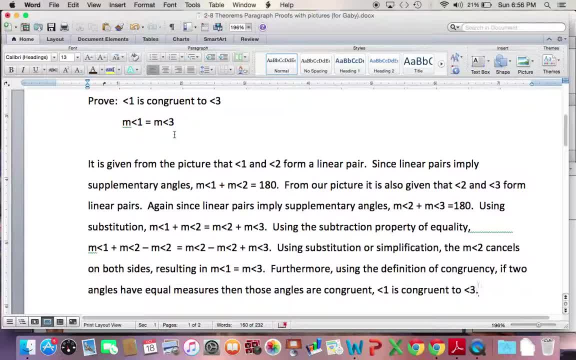 Now, since we've proved it together, it's fair game. We can go ahead and apply it to proofs, which you'll see more tomorrow. And remember we always use an if-then statement in our proofs, so an example of this as an 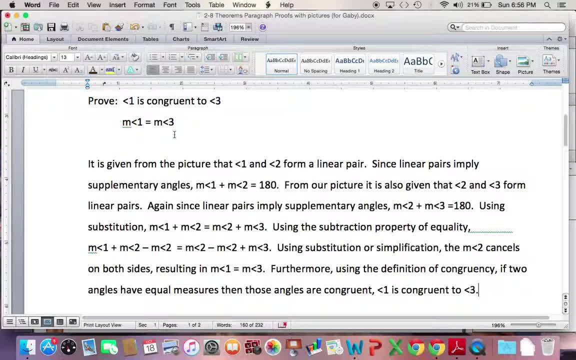 if-then statement would be vertical angle. So if two angles are vertical angles, then they are congruent. That would be an example of our if-then Okay. so, using this same technique, we're going to go ahead and look at number 5, which 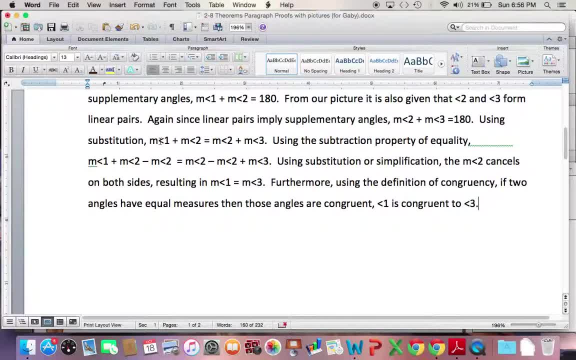 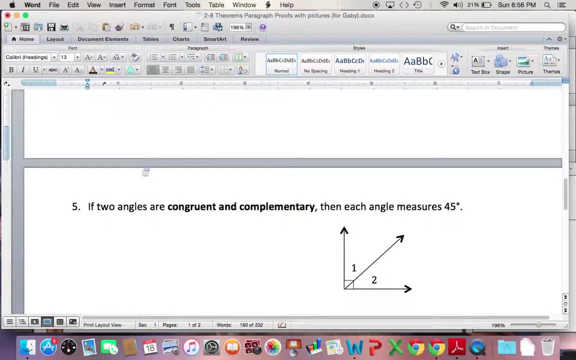 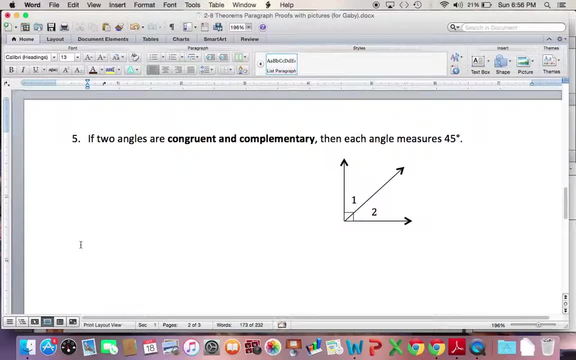 is similar to the second paragraph, proof from your homework from earlier last week. So let me just put this on the next page so you can see it all together. So notice and let's get some space. Notice you have: if two angles are congruent and complementary, then each angle measures. 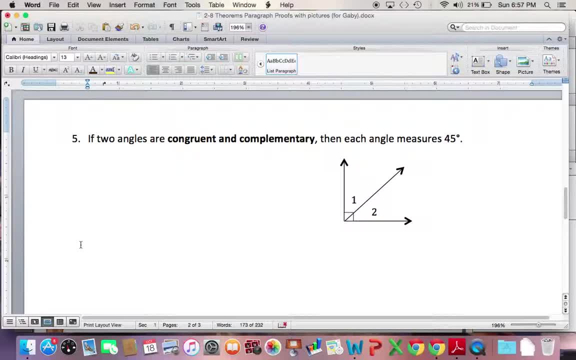 45 degrees. So again on your paper, you don't have anything drawn, You don't have your if-then given to you, your conditional statement given to you as what you're given and what you're trying to prove. We need to do all of that. 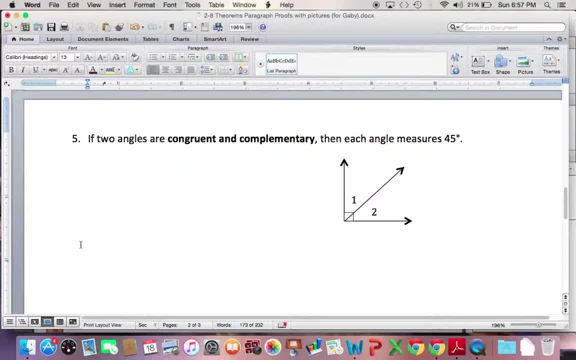 So go ahead and draw in this picture that represents this theorem. Okay, so the next piece that we need is: we need what we're given and what we're trying to prove. So let's go ahead and type that out. So we have what we're given is, according to our picture, angle 1 is congruent to angle. 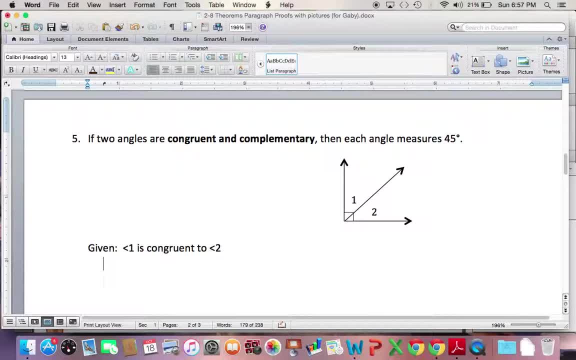 2. We're also given that angle 1 and angle 2 are congruent, Okay, Okay, So the two angles that we're given are complementary And we can tell that from our picture because we have this right angle notation, this little. 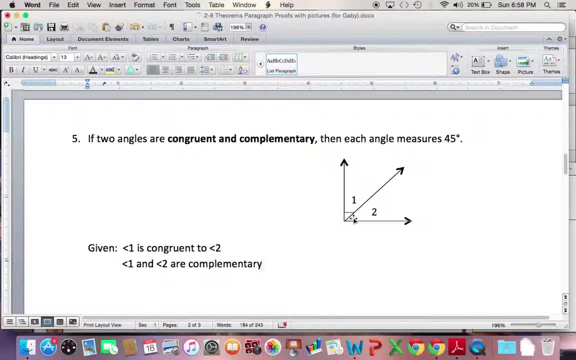 box here. If we didn't have that, although those two angles look complementary, we would not be able to say that. Remember, you can't assume that unless the notation is there for you. Okay, So what is it that we're trying to prove? 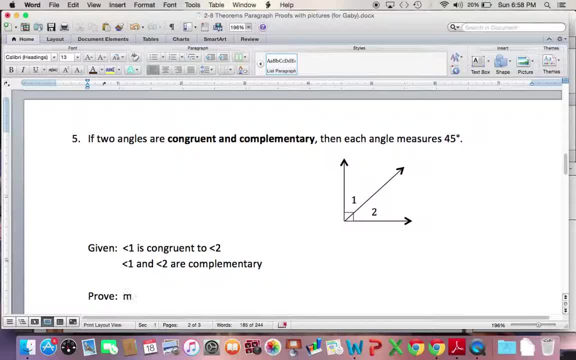 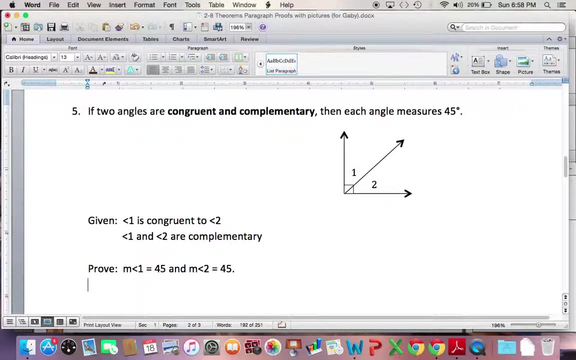 So we're trying to prove that the measure of angle 1 equals 45 degrees And the measure of angle 2 also equals 45 degrees, And we're going to tackle this the same way. We're going to kind of think of our game plan and then type it up. 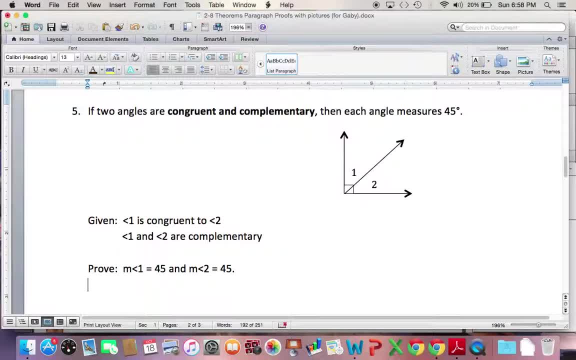 So first let's think this through. We know angle 1 and angle 2 are congruent, so therefore we know their measures are equal. So these two angles, we know they're equal by the definition of congruency. We also know, by the definition of complementary, that the sum of angle 1 plus the sum of the 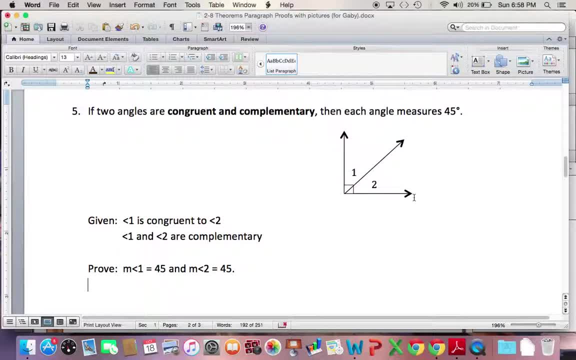 two angles equals 45 degrees. So the sum of the two angles- meaning the measure of angle 1 plus the measure of angle 2, is going to equal 90 degrees. So since we know the two angles are equal and that the sum of the two equal 90,, we can: 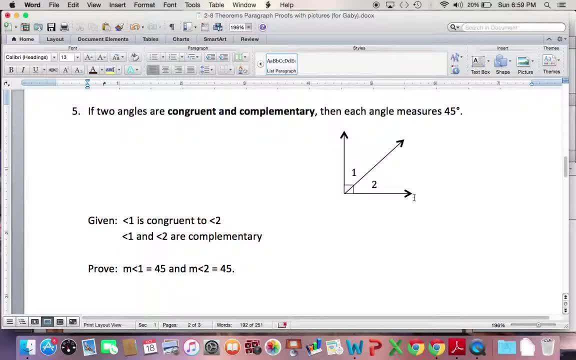 substitute the measure of angle 1 in for the measure of angle 2. And we'll end up with 2 times the measure of angle 1 equals 90. Then we can go ahead and divide on both sides and we get the measure of angle 1 equals 45.. 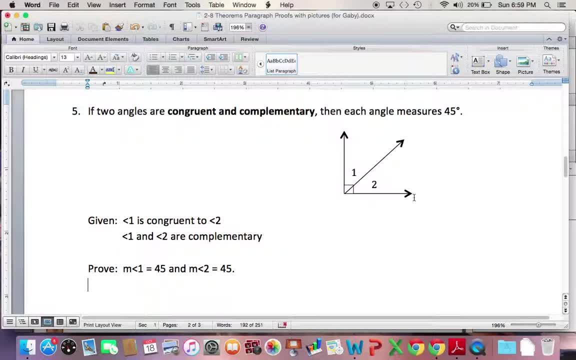 And then because we know the measure of angle 1 equals the measure of angle 2, we can say the measure of angle 2 is 45. So it's kind of- I know I kind of went through that fast and there's no visual to kind of help you. but 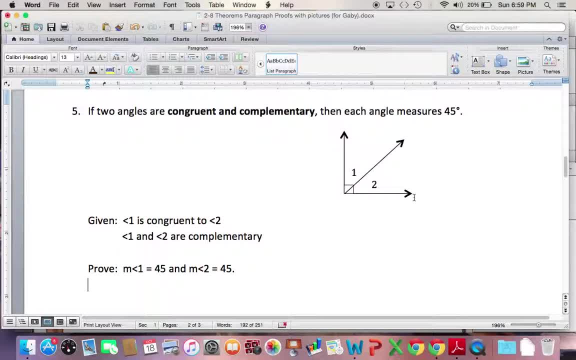 let's go ahead and type this up and you'll see. if you didn't understand the game plan right away, you'll kind of see it unfold as we're typing, or as you're writing and I'm typing, So let's begin. So it is given that angle 1 is congruent to angle 2.. 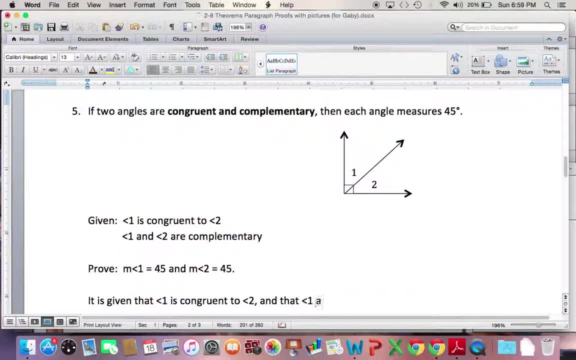 It's also given so we can say: and that angle 1 and angle 2 are equal. So it's also given so we can say: and that angle 1 and angle 2 are equal. So it's also given so we can say: and that angle 1 and angle 2 are equal. 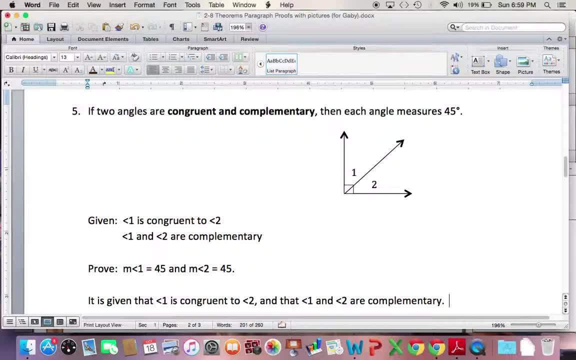 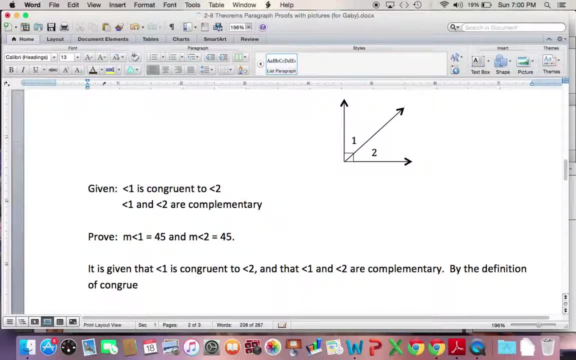 So it's also given, so we can say: and that angle 1 and angle 2 are complementary. We know by the definition of congruency-oops-that if two angles are congruent, then their measures are equal. Right, Right. 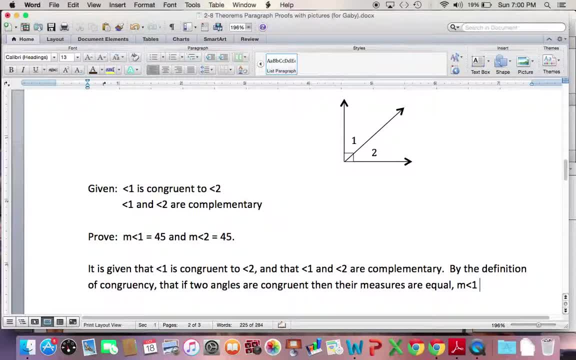 Yeah, So equals the measure of angle 2.. We also know, by the definition of complementary angles, whose angles who are complementary have a sum of 90 degrees. So pretty much, if two angles are complementary, we know the sum of the two angles: the measure of angle 1 plus the measure of angle 2,. 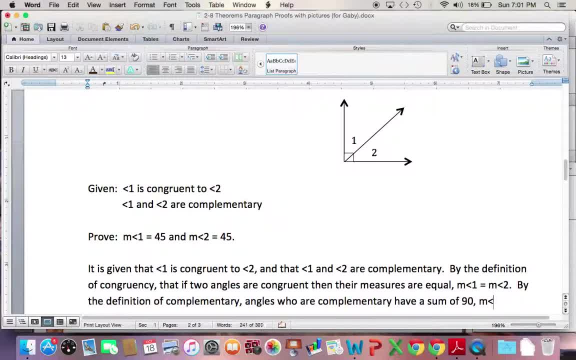 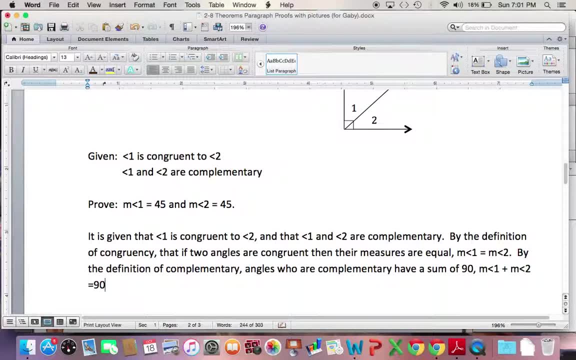 equals 90 degrees. So, furthermore, measure of angle 1 plus the measure of angle 2 equals 90 degrees. Again, I'm just going to kind of space this out so you see it all together. Sometimes it's a little challenging on Word to go back and look. 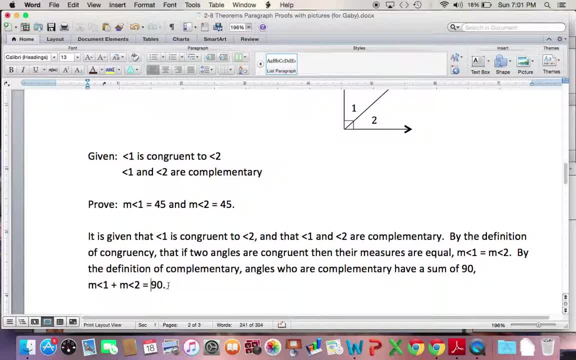 when it's not all on one line, like we're used to writing in our handwriting. Okay, so we went ahead and we stated all our givens and we converted them to equality statements, which is what we're going to need. So we know we can use substitution. so 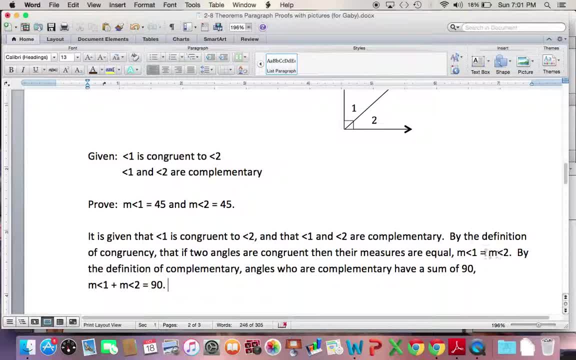 because the measure of angle 1 up here, the measure of angle 1, equals the measure of angle 2, I can substitute the measure of angle 1 in for the measure of angle 2 here. So using substitution we can say the measure of angle 1. 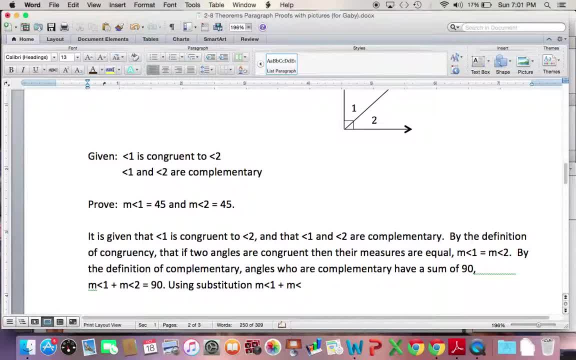 plus the measure of angle 2..1,. excuse me, we're substituting measure of angle 1 in for the measure of angle 2, equals 90 degrees, Which simplifies to 2 times the measure of angle 1: equals 90 degrees. 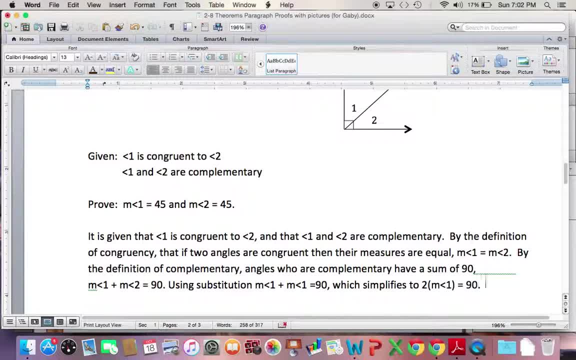 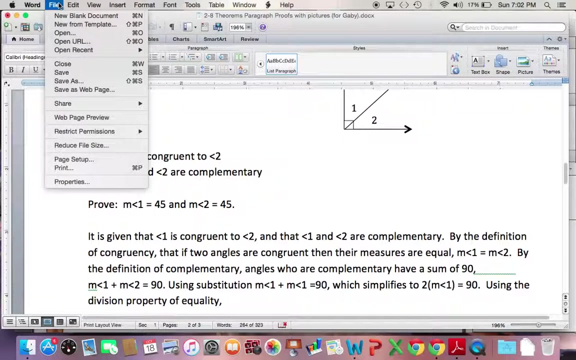 So, using the division property of equality, we can divide by two on both sides. so I'm going to need to insert an equation for this. you guys would just, you know, draw your division bar and divide by two on both sides. so just bear with me for a second. 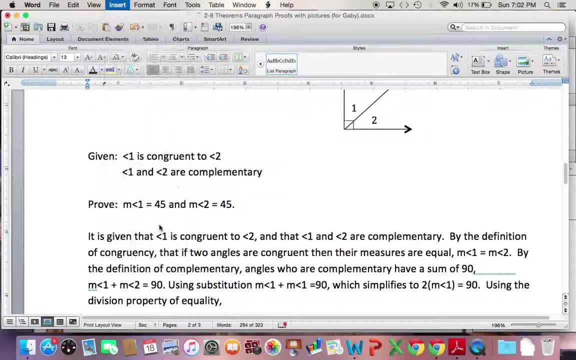 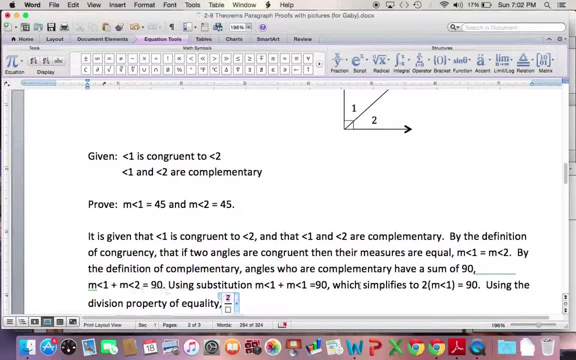 I need to insert an equation here and I need a fraction to show what's going on. so I have two times the measure of angle. one is being divided by two and we know that whatever we do to one side of the equation, we have to do to the other. so 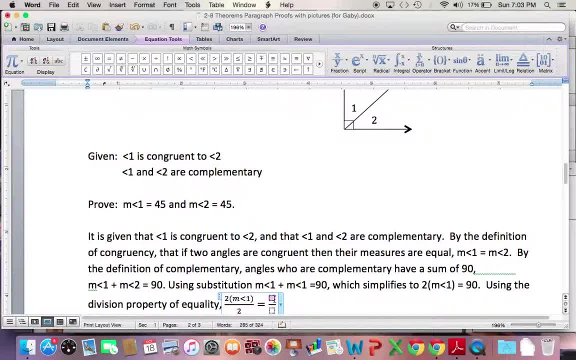 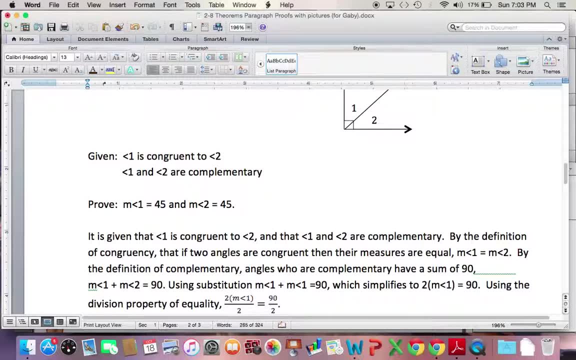 again on this side I'm going to have 90 divided by 2. and again you guys, you know you're writing this out, so it's much easier for you to just show the division. I had to use a fraction in word to go ahead and do that. let me just scroll. 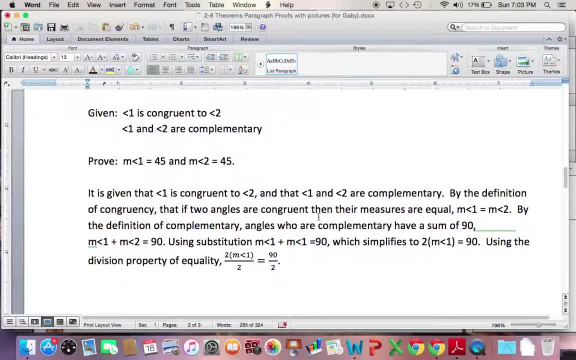 forward, so we have a little bit more space. okay, so now we know this: simple substitutes, substitutes or simplifies. in other words, sometimes simplifies makes more sense to us, but we know that we can use the substitution in place of simplification. so this substitutes or simplifies to the measure of angle one. 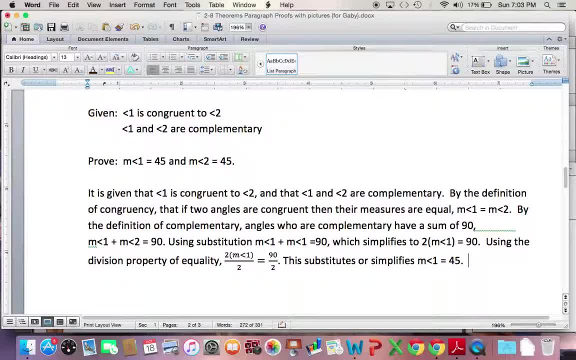 equals 45 degrees. now, looking back here we know the measure of angle one equals the measure of angle two. so we can use substitution and substitute 45 in for the measure of angle one here, saying that the measure of angle two equals 45 as well. so, as previously stated, since the measure of angle one equals the measure of angle two, 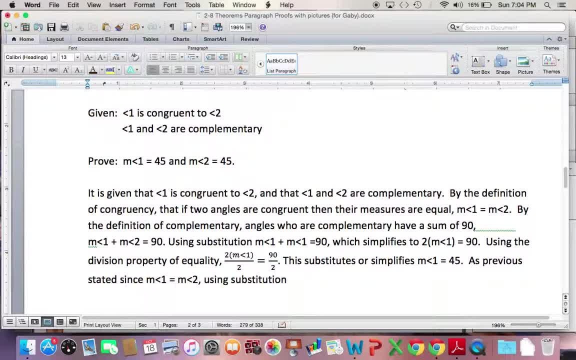 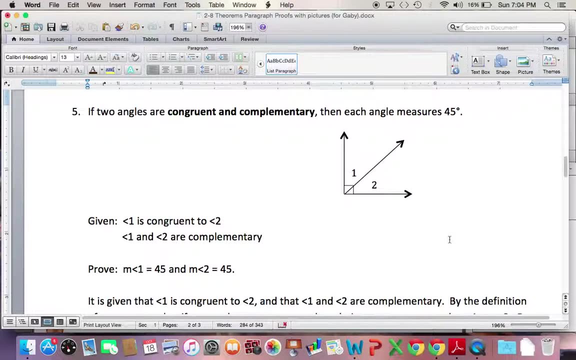 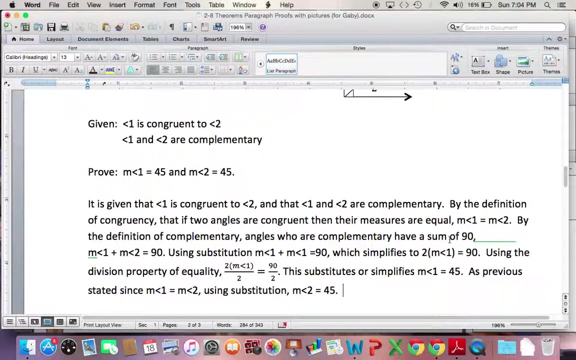 using substitution measure of angle two also equals 45 degrees. so again, because we've now proven this, this theorem, that if two angles are congruent and complementary, then each angle measures 45 degrees. tomorrow you'll notice in your when you're practicing your proofs in class and for homework. 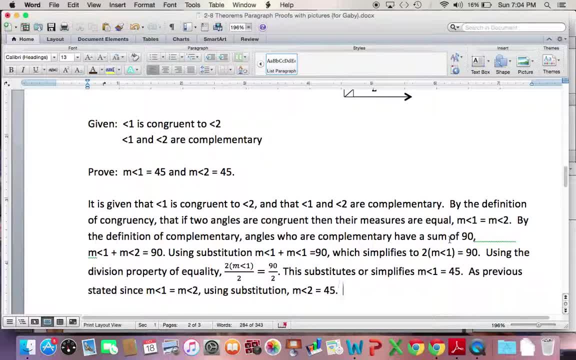 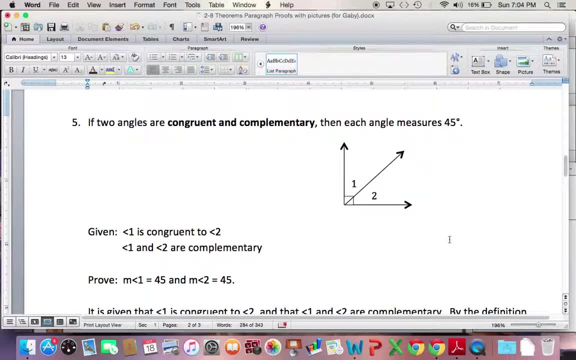 you can now use this. it's fair game. So for the remainder of the period you're going to use this technique how: first we drew our picture to represent our conditional statement, Then we transferred our conditional right, We wrote our hypothesis as the given and our conclusion as what we're trying to prove.